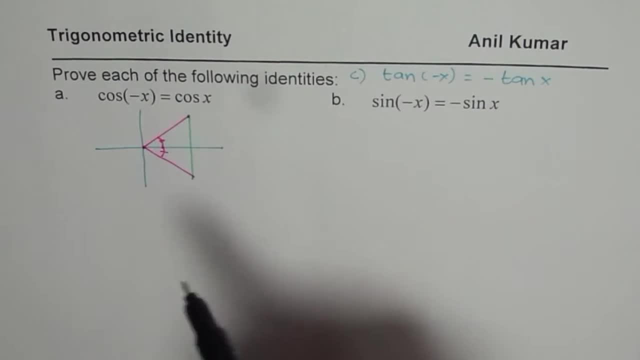 Of the same point in different coordinates, right? So you can see if I take two points. let us say p and its image, p dash, reflected on x, for example. In that case, coordinates of p will be x- y and the coordinates of p dash will be x minus y, since it is going downwards. Do you see that? So those are the coordinates, And op is r. let us say, right, Which is: 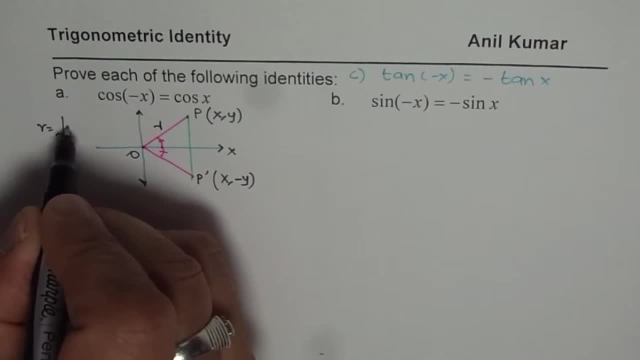 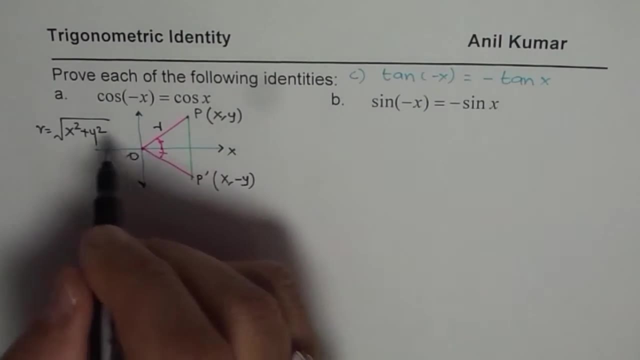 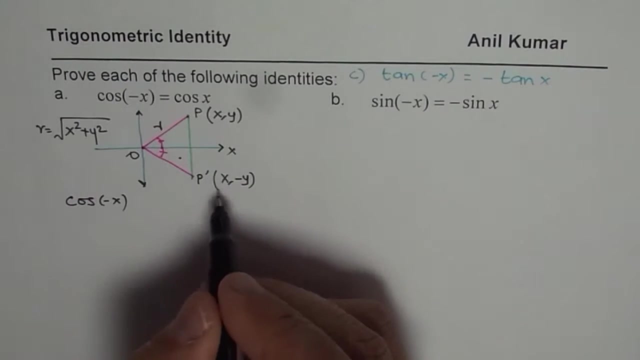 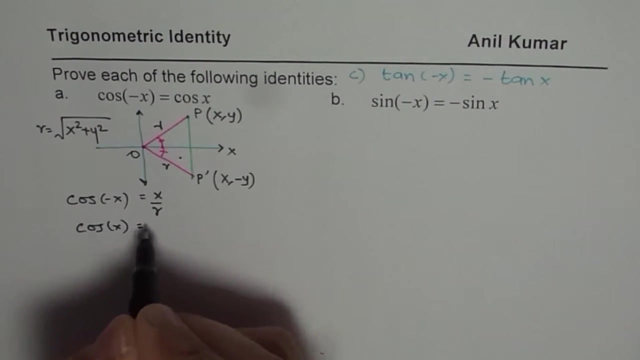 where you know r is equal to square root of x square plus y square, which is always positive. Now, what is cos of minus x? Cos of minus x is- we are working in this triangle- will be x over r, right, So it is x over r. And cos of x is also x over r, right, So they are both equal. So you can say: 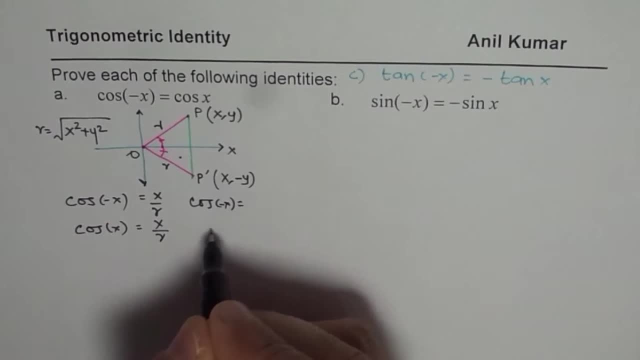 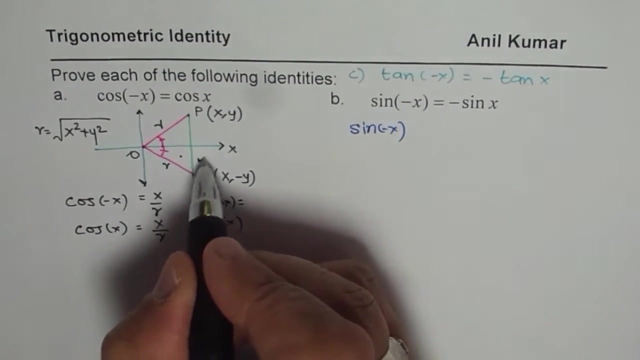 that cos of minus x equals to cos of x, correct? So both are equal. If you do the same thing for sin, then what do you get? So I am not sketching it again, but let us do the same thing for sin. So in the case of sin, sin of minus x will be. you are working on this particular triangle. So y values minus y, right? So sin of minus x is minus y. 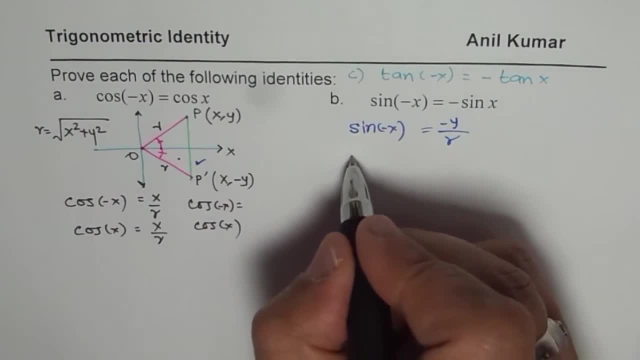 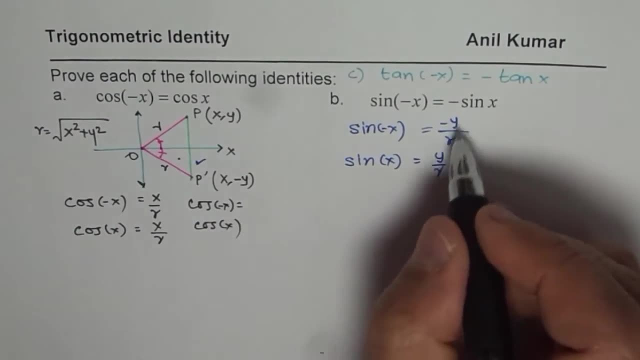 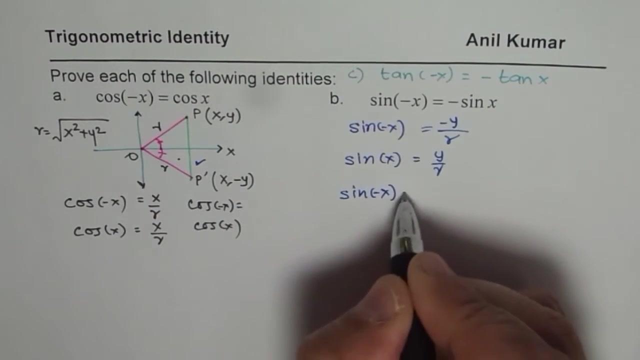 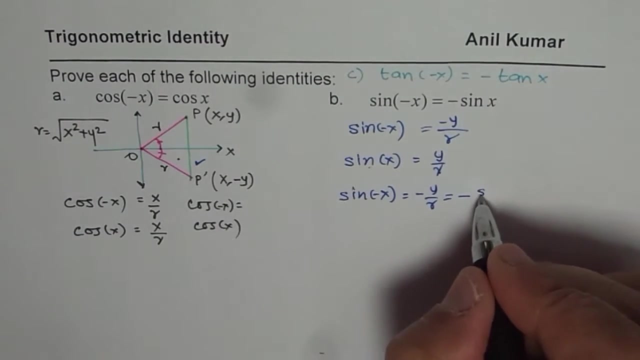 over r, whereas sine of plus x is this y over r. and from here, you know, you can place sine of x, sine of minus x, which is minus y over r, as equals to minus of y over r. instead of y over r, let us write sine x sine x, correct? so that is what we get. so sine of minus x is minus sine x. 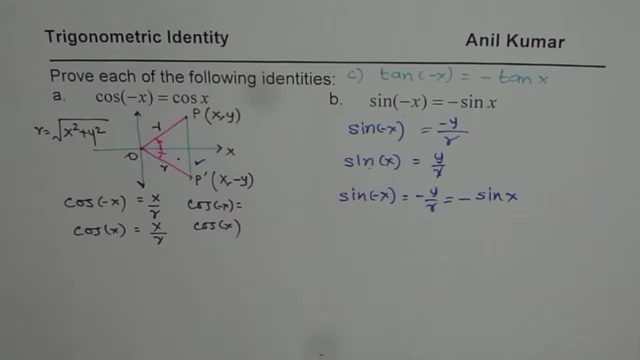 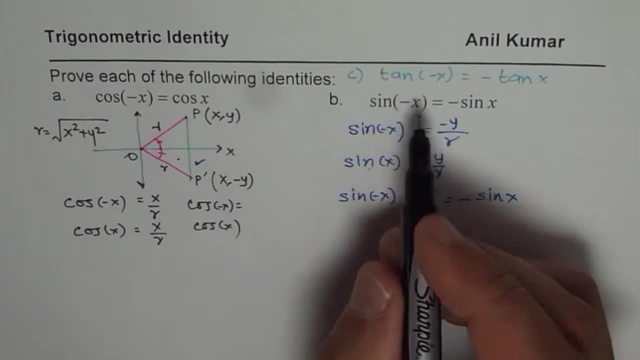 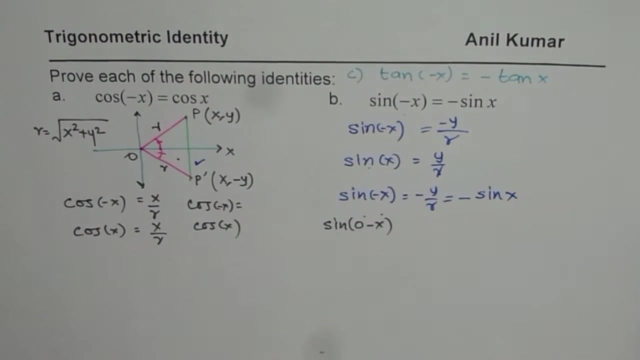 that is one way of doing it. you have also studied compound angle formulas, right? so we can use compound angle formulas to prove this also. consider sine of zero minus x, for example, correct, both in degrees, for example. is it okay in that case? if you expand it, what do you get?